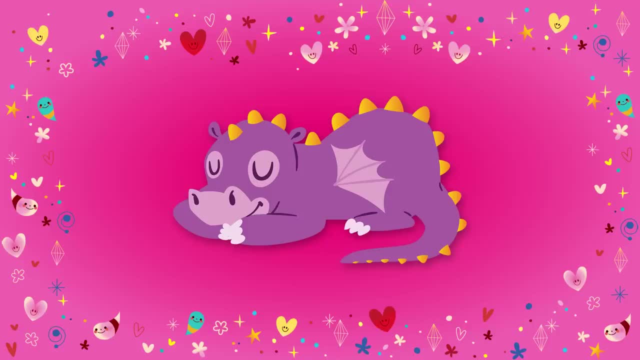 As you learn about them, maybe you'll see how life for the dragons is quite similar to the way we live. Mummy dragon was called Delilah, Daddy dragon was called Doug, And they had a little girl dragon called Dina. They lived together. 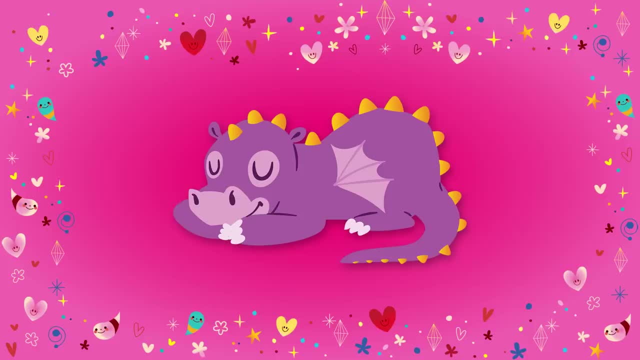 On a mountain covered in flowers and grass And had a lovely mossy cave where they ate together and slept. Nearby was the waterfall and pool where they would take a shower or bath Every day. Mummy Delilah and Daddy Doug went out to work. 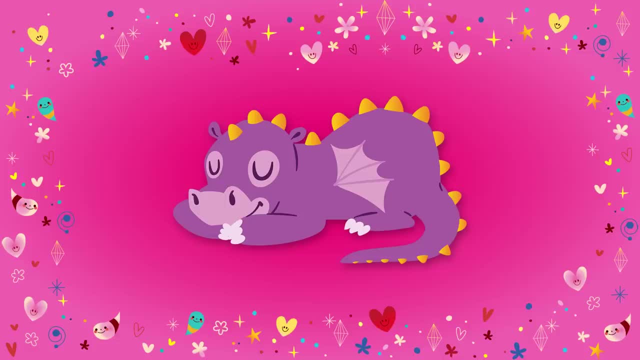 They had a restaurant called The Flame Grill where they prepared delicious barbecue vegetables and toasted marshmallows for dessert. It was hugely popular with all the dragon families in the area, So they were very busy most days, and sometimes the evenings too. Dina spent her days at dragon school practising her powers. 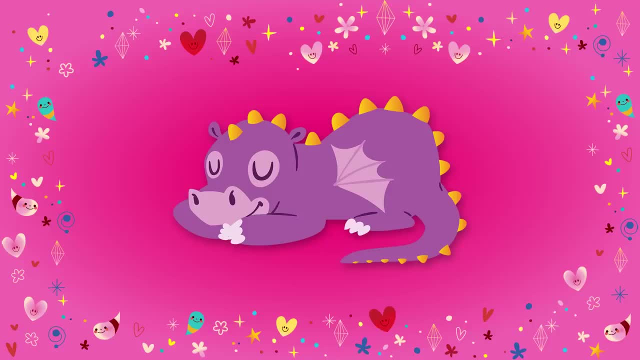 Exercising her wings with some flying, Drawing cloud pictures in the sky, Changing colour to camouflage herself And learning how to control her fire Breathing. There was so much to learn and practise. Sometimes Dina found it hard and frustrating, as she just wanted to be good at everything. 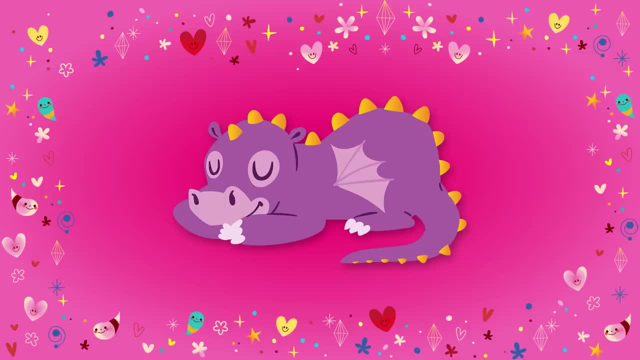 right away And lately, when she got angry at things not going her way, she would end up setting fire to everything around her. That didn't help at all, But she kept on trying And it only made her feel upset at the damage she'd caused. 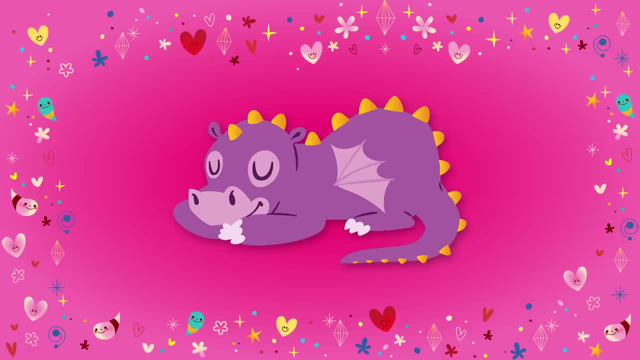 Dina was learning how powerful her feelings could be, But it was happening more and more often. Losing a game of Dragonopoly, Not making her cloud picture just as she hoped, And even having trouble making her bed in the morning tipped her over the edge and 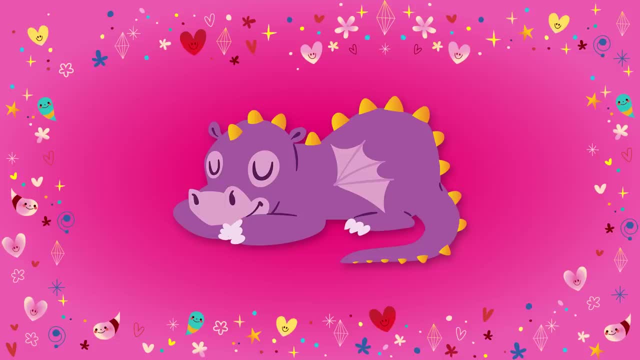 she set fire to her pillow. All this frustration was getting her down. One day Miss Blaze, Dina's school teacher, took Dina aside after lunch. She had seen how Dina was struggling to cope with her fiery feelings and wanted to help. 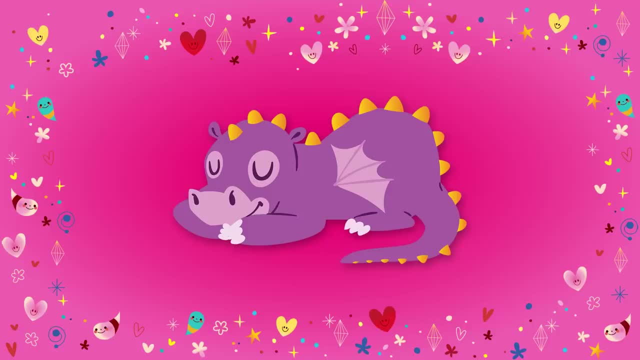 Miss Blaze explained how a dragon's brain and body need time and patience to learn how to do things. She gave Dina some very special advice. The best thing a young dragon can do is learn how to use your breath to steady the fiery feelings we all have. 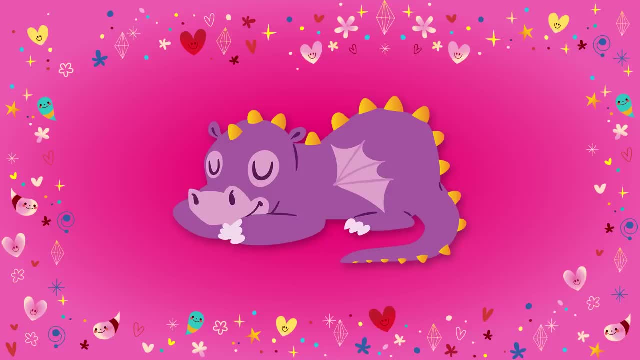 Dina decided to give it a try. Burning everything to a crisp wasn't helping, And she needed to do something. So she started practising calming her breath down Every day, Spending just a few moments closing her eyes, Noticing her breath. 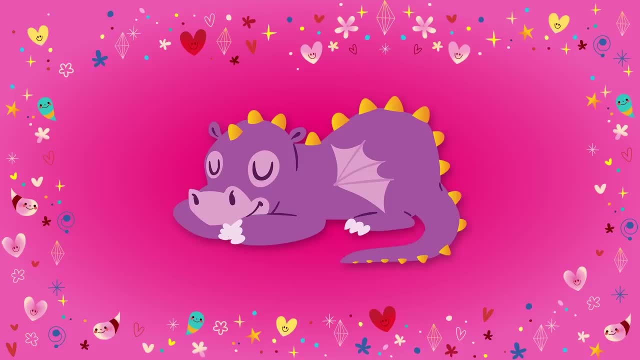 The in And the out And slowing it down. After a minute or so of doing this, she felt calm. Her mind would feel clearer And on opening her eyes she felt good, Like her body and mind were thanking her for being calm. 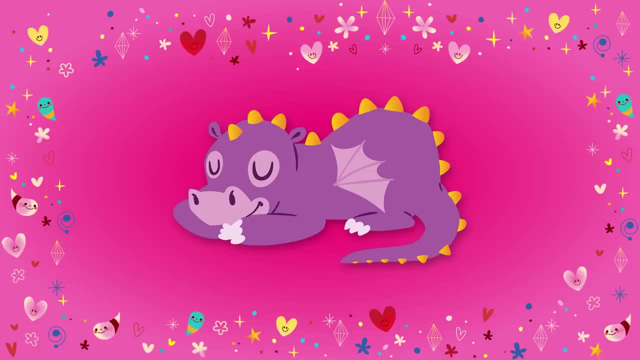 Like her body and mind were thanking her for being calm, Like her body and mind were thanking her for being calm, Thanking her for being kind to herself, Thanking her for being kind to herself. After a week of practising her daily breathing exercise, Dina's parents noticed how their 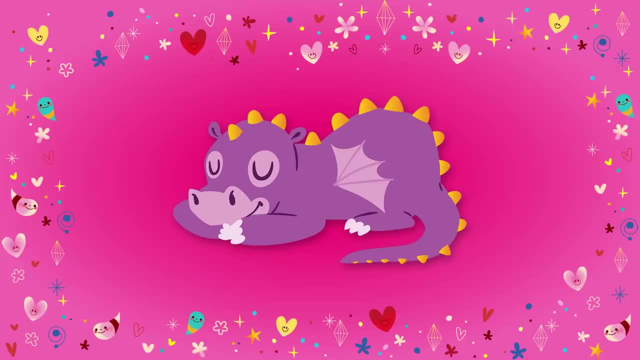 daughter seemed happier, somehow Calmer. They knew she'd been having trouble at school, That her frustration could send everything up in flames And that she hadn't really been sleeping well. But something had changed. during bath time, when Doug asked Dina how everything was going and Dina explained how. 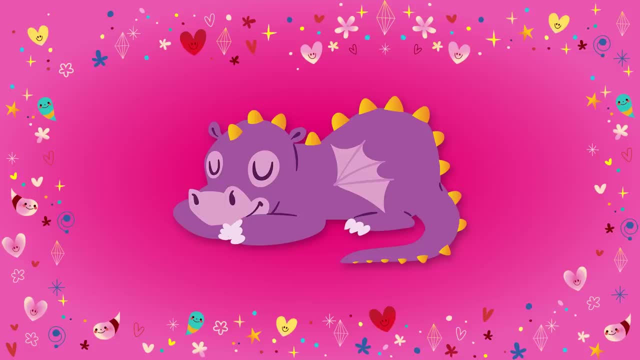 she'd been learning to calm her breathing, that she was noticing when a spark of anger would appear, when she found something hard, and that with the little breathing practice every day, she just felt better in herself, somehow more in control of her feelings. Doug was so proud of his little dragon baby girl. she climbed out of the bath and he wrapped her up. 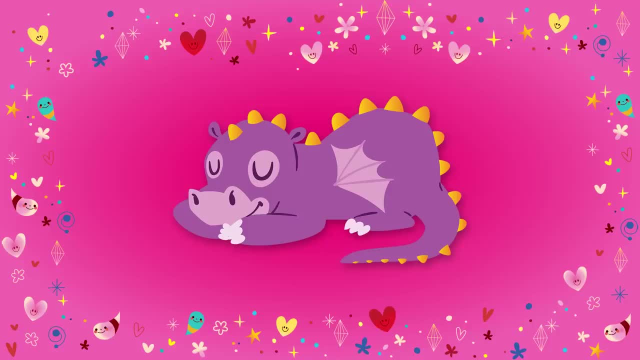 in a towel, hugging her tightly While she changed into her pyjamas. Doug quietly shared Dina's news with Dina's mummy, Delilah, who was just as proud and relieved that their daughter was going to be okay. That night Dina was in the bathroom with her baby girl. 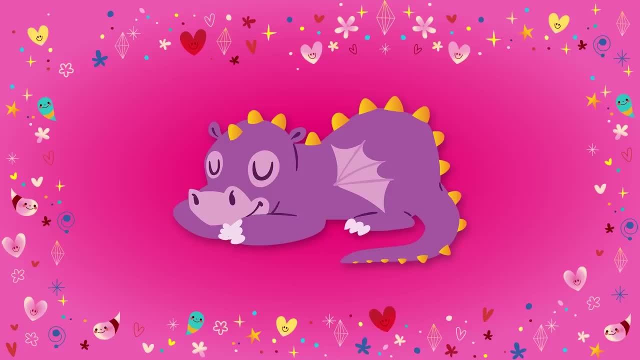 Dina's mum Delilah, who was just as proud and relieved that their daughter was going to be okay That night. Dina's mum Delilah, who was just as proud and relieved that their daughter was going to be okay. Dina snuggled up in her mossy squishy bed with her new pillow, feeling ready for a sleep. 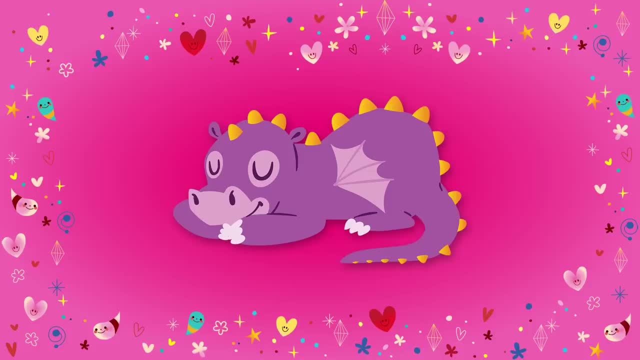 Nowadays, she looked forward to sleeping as she felt stronger every day when she woke up, and that was the time she chose to do her breathing exercise every morning. Let's find our sleeping dragon position now, our body relaxing: our legs, arms, our face, our long back and tail. if we're being dragons, relaxing and getting heavier and heavier. 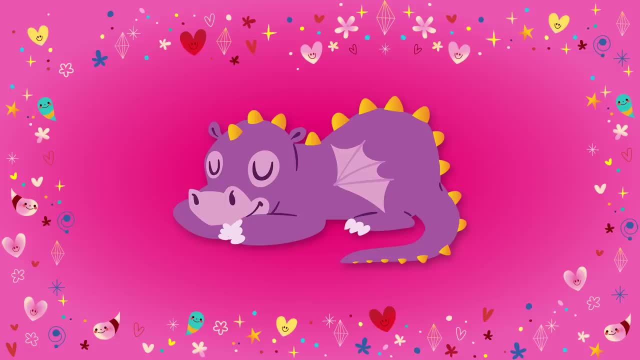 As sleepiness begins, with each breath out, little wisps of smoke puff from our noses. another day, as sleepiness begins with each breath out, little wisps of smoke puff from our noses. another day. learning a bit more about ourselves comes to a close, and the night wraps us up in a cloak of stars, resting easy like a sleeping dragon. 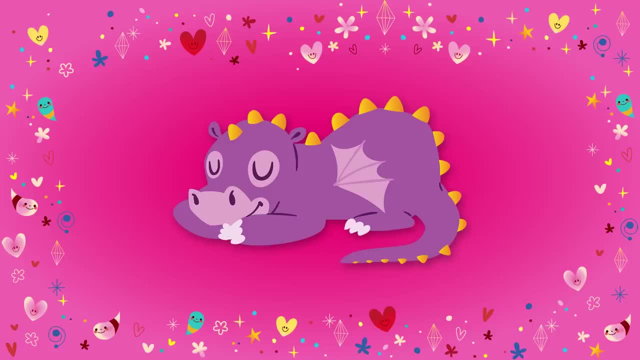 and the night wraps us up in a cloak of stars, resting easy like a sleeping dragon. If now is sleep time, then I wish you a good night. If now is sleep time, then I wish you a good night. If it's not time for bed yet, then slowly start to come back.